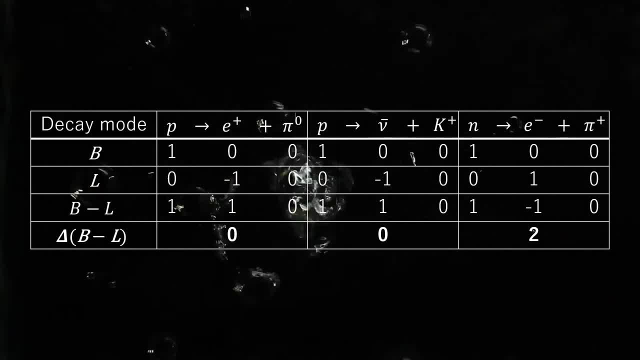 In high-energy physics, B-L is the difference between the baryon number and the lepton number. This quantum number is the charge of a global gauge-U-1 symmetry in some grand unified theory, gut models. Unlike a baryon number alone or lepton number alone, this hypothetical symmetry would not be broken by chiral anomalies or gravitational anomalies. 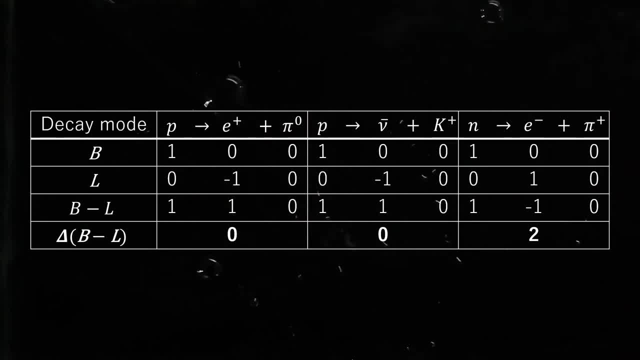 as long as this symmetry is global, which is why this symmetry is often invoked. Quarks and leptons are indistinguishable in any 4D gut and both the baryon and lepton number are not conserved. This leads to baryon number violating nucleon decay. 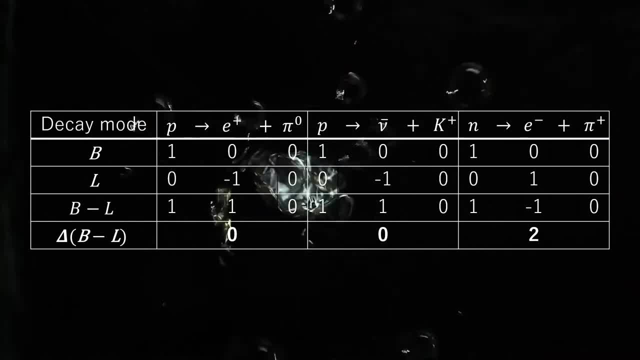 In addition to the baryon number violation, lepton number violation is also required for nucleon decay, since in the standard model leptons are the only free fermions which are lighter than nucleons. The lowest dimension operators relevant for nucleon decay are violating dimension 6-4 fermion terms in the standard model. 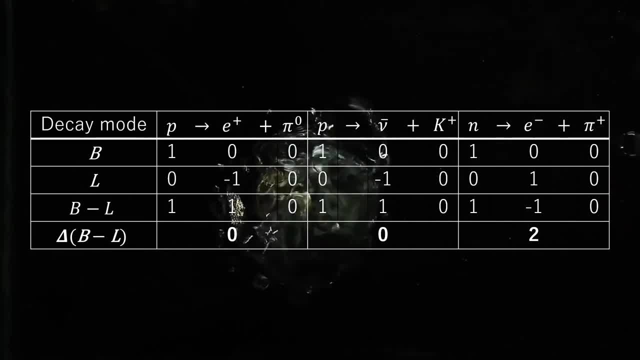 and all baryon-violating operators with dimension less than 7 preserve b-L. One hypothetical example is proton decay, where proton would decay into a neutral pion and positron. This proton decay conserves b-L even though it violates both lepton number and baryon number. conservation: 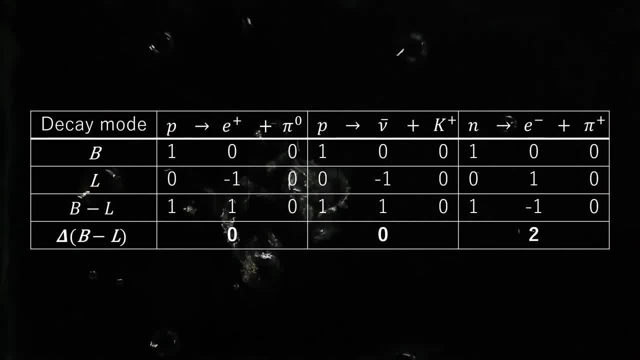 On the other hand, one can consider b-L violating phenomena. They are interesting in their own right and may also be relevant to baryogenesis. The relevant operators have higher mass dimension than the familiar dimension-6, b-L-violating operators. They may be predicted in S-O-10 guts with an intermediate scale. 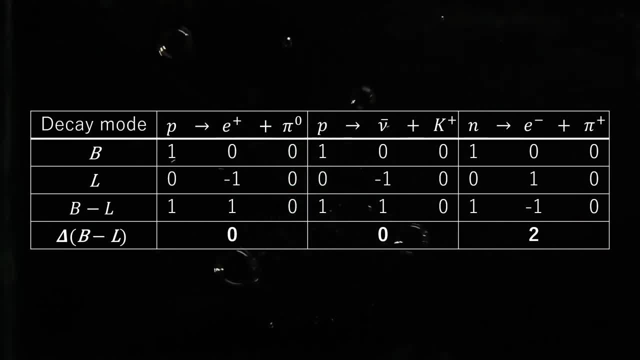 at which baryogenesis can be observed. First, one may have nucleon decays with delta-b-L equals 2, such as a neutron would decay into a positively charged pion and electron. Second, there are neutron-anti-neutron oscillations. 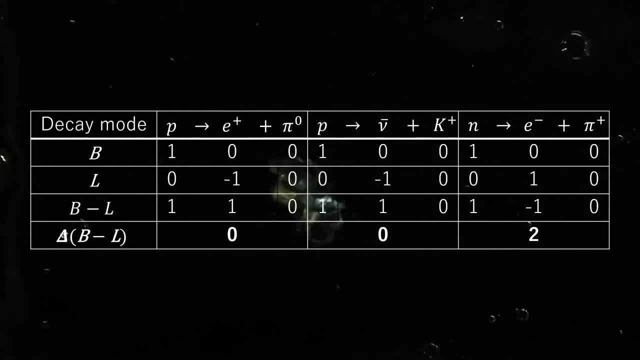 which are induced by delta-b-E equals 2 dimension-9 effective operators in the standard model.